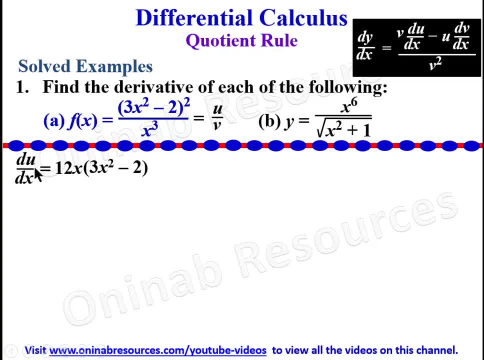 1 gives 1.. This is still the same thing. Therefore, the u dx is 12x into 3x squared minus 2.. Then we go ahead to find the v dx. Here the v? dx is 3x squared. 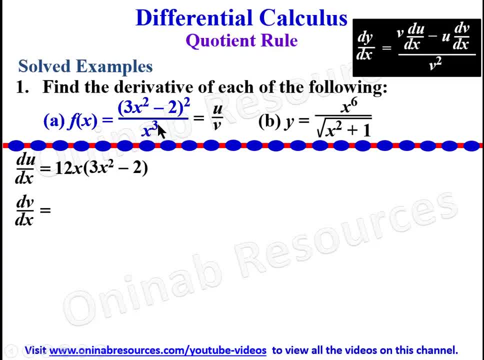 If you multiply by the power, that will give you 3x cubed. Reduce the power by 1. It gives 3x squared. Now we go ahead to find the y dx We substitute into this formula: We have v here and our v is x cubed. So we have x cubed, The u dx, Our du dx is 12x, into 3x squared. 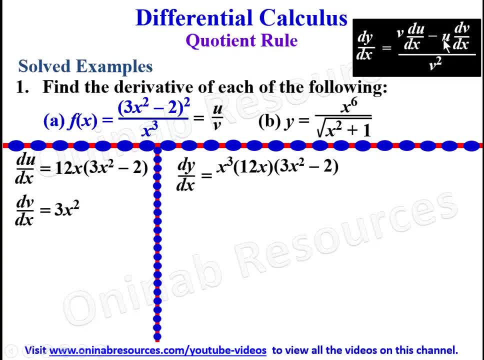 minus 2.. Then we have minus u. Our u is 3x squared minus 2 all squared. The v dx is 3x squared. We have 3x squared all over v squared. v squared, that is x cubed squared. So we go ahead to. 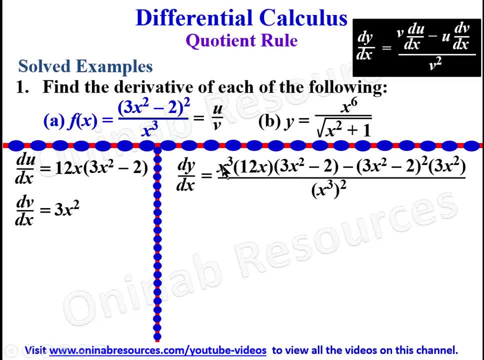 simplify the numerator and denominator: x cubed times 12x will give us 12x to the power of 4.. Then we have the brackets Minus 3x squared into 3x squared minus 2, all squared, Then over x raised to the power of 6. This 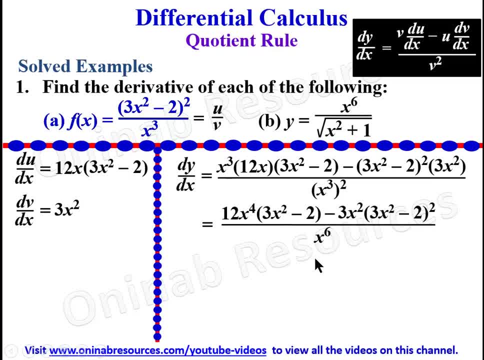 is 3 times 2, which gives x raised to the power of 6.. Now we can factor out the numerator. I look at 12x squared and 3x squared. 3x squared is a factor of 12x squared. So we have that. 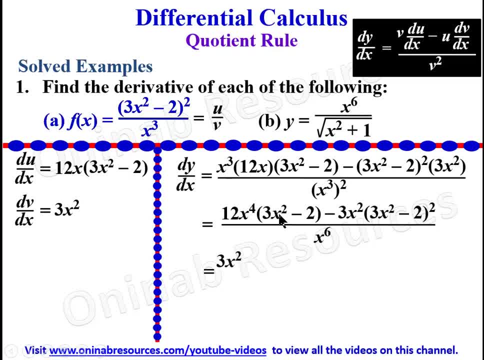 factor there, 3x squared. And we look at the brackets, This is 3x squared minus 2 to the power of 1.. 3x squared minus 2 to the power of 2.. So this 3x squared minus 2 is a factor. 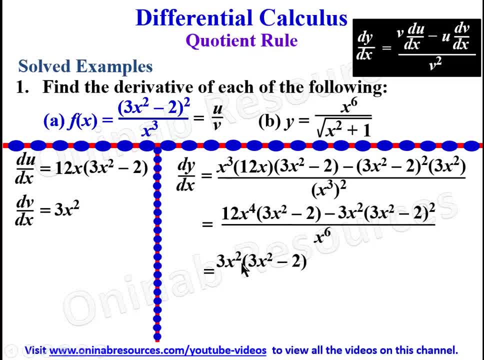 So we bring out 3x squared minus 2.. Now we factorize 12x 4 divided by 3x squared, We give you 4x squared. These 3x squared minus 2, divided by 3x squared minus 2, gives us a. 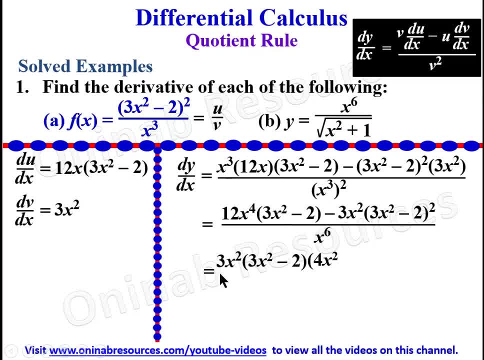 1.. So we are done with that first part. The second part, 3x squared. here. divided by this, 3x squared is 1.. We're你说 x, vaccines of v, And we have the third day. This is 3x squared. 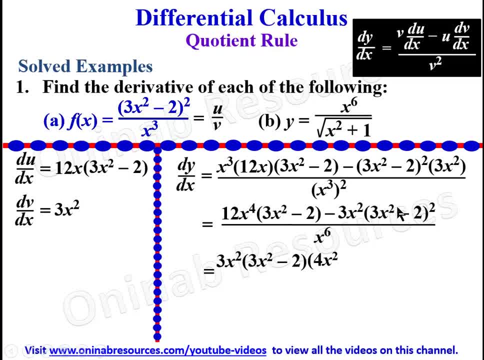 minus 2.. And now we have the third day, This number off the denominator, word 2 and all expected times and times. So once we've included y and y, We're now done. The third day is a continuous. we don't have business there. then, 3x squared minus 2, all squared divided by 3x squared minus 2. 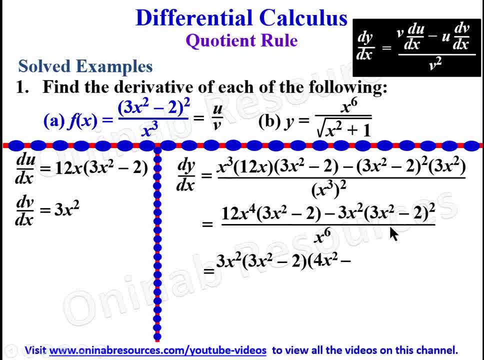 so it will go with 1. so we'll be left with 3x squared minus 2. bringing it here, this is a. multiplied by this we give us a minus 3x squared. this minus multiply minus will give us a plus 2, all over x to the power of 6.. this goes with. these will be left with x raised to power 4. the 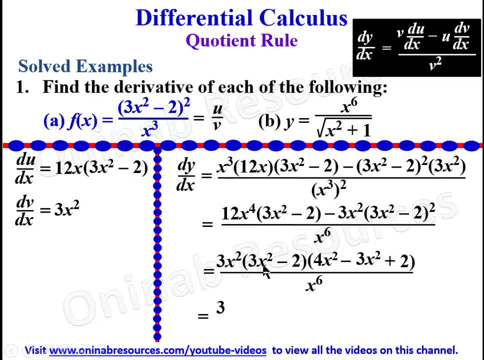 denominator will only be left with 3 here and 3x squared minus 2. simplifying this: 4x squared minus 3x squared is x squared then plus 2 over x raised to power 4.. this is the derivative of the function in a, so that is f, prime of x, or the y the x. so we go to problem b for problem b. 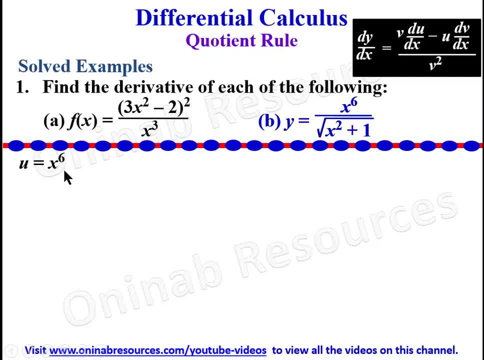 um, we let u be equal to x, raised to power 6 and u the x, there will be 6x to the power of 5, multiplied by this 6. reduce the power by 1, so i have 6x to the power of 5 and our v is x squared. 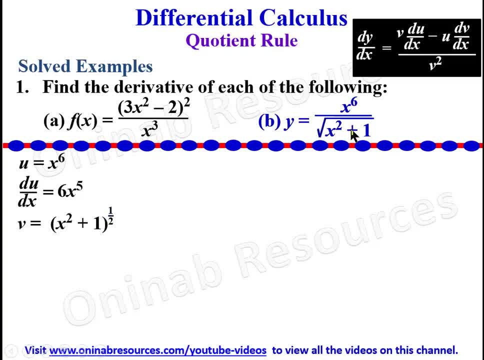 plus 1 to the power of half. i've written that in index form, so differentiating this. we have dvdx. differentiate what we have inside the brackets. that's 2x multiplied by the power, half it will give x bring the power. reduce this power by 1. that's half minus 1 gives negative half. 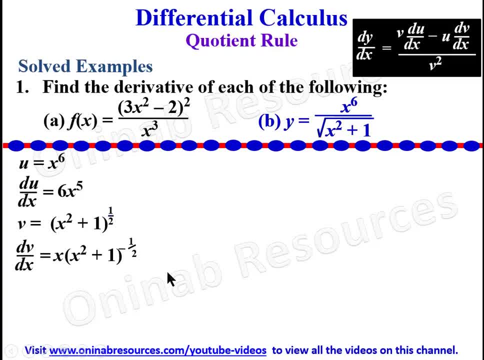 so we have it to the power of negative half. then we now go ahead to find the y, the x, using this uh rule. our v is square root of x squared plus 1, and the u, dx is 6 x to the power of 5 minus u. 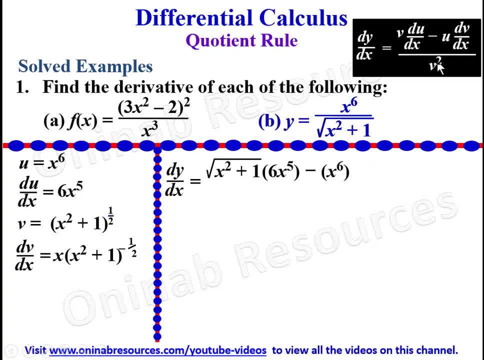 our u is x to the power of 6 multiplied by dv, dx. but this is this. we have it as this. then, over v, over square root of x squared plus 1 squared, squared it, this is v squared. now we go ahead to simplify this: 6x to the power of 5. 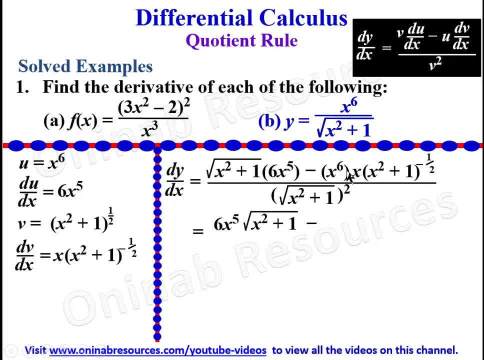 root, x squared plus 1 minus x, raised to power 7 into x squared plus 1, all to the power of negative half. then divide by the square root. here we remove this square, so i'll be left with x squared plus 1.. um, we can go ahead to still simplify. uh, x 5 is a factor of this. 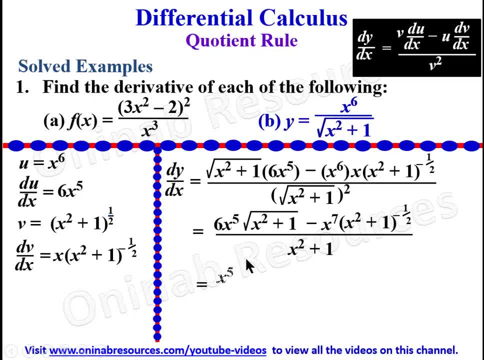 so i have x to the power of f5, and here x squared plus 1 roots um. yeah, this is a factor, this is a factor. it's a factor we can now factorize here. factorizing 6x to the power of 5 divided by x to the power of 5 will give: 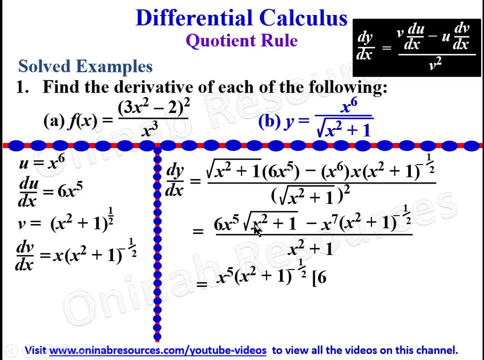 us a six, and this is x squared plus one to the power of half. dividing it by this, we give us a x squared plus one. yeah, it's just like having m to the power of half divided by m to the power of negative half. since it is division, the half here will be plus half there will be. let it. 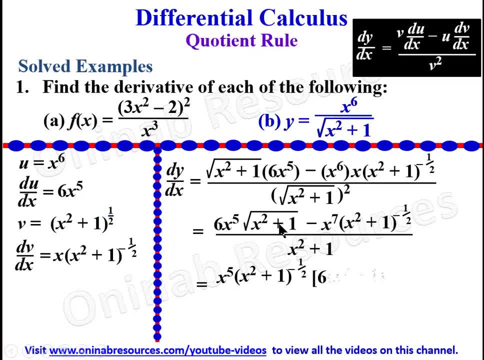 m to the power of one, which will just give us x squared plus one, then minus x to the power of seven. divided by x to the power of five, we give us a x squared, and since this, divided by this, will give us one, that's the numerator over x squared plus one. um, we go ahead to simplify this. 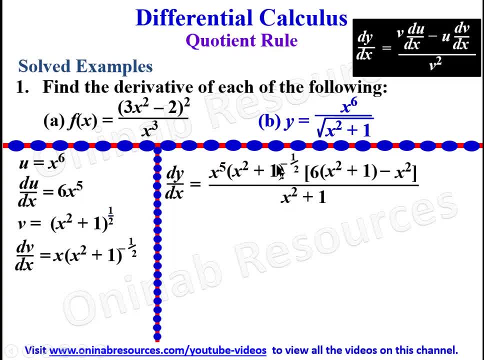 go ahead to simplify this, we still maintain these first two factors. six x squared plus six- here this is x squared- will go with this. negative x squared will be left with five x squared plus six plus x. then over the denominator there, um, now, uh, i want to rearrange and see if this can divide this. this is x to the power of five into five x. 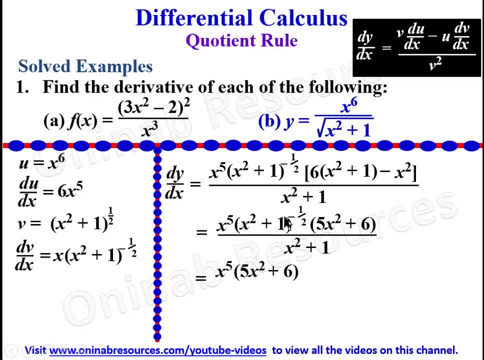 squared plus six. if i take this to be m, this x squared plus one to be m, this will be m. so i'll be left with m to the power of half, divide by m to the power of one, and this is m to the power of negative half. 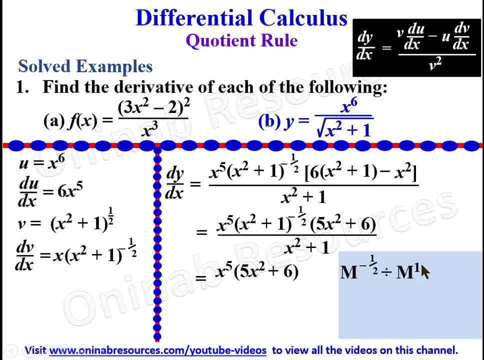 uh, negative half minus one will give us negative three over two. so i will have my answer as m to the power of negative three over two and i can write this as fraction. writing it as fraction, i have one over square root of m cube square root. this denominator will form the square root.